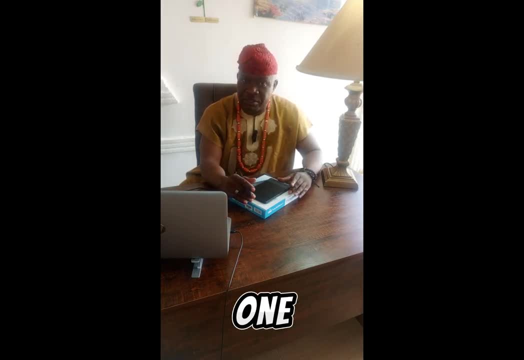 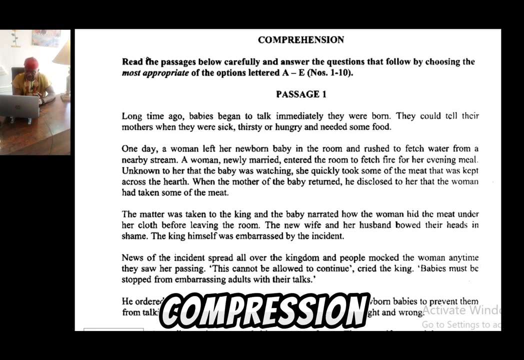 going to be an exciting class. It's going to be a helpful one because it will help you ace the exam- the English aspect of it. So, if you're ready, join me in the class. All right, we are going to start with the comprehension passage. The instruction says: 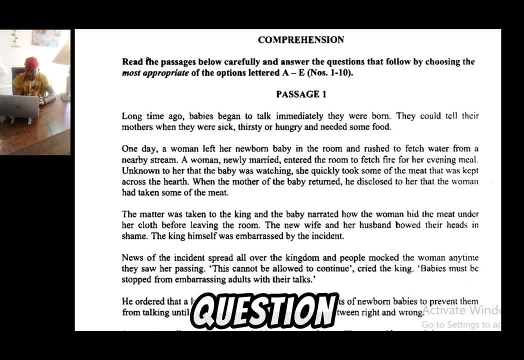 read the passages below carefully and answer the questions that follow by choosing the most appropriate of the options later. A to E: This comprehension passage takes care of questions one to ten. It's always very good to read the instruction before you take any task, because it guides you and lays 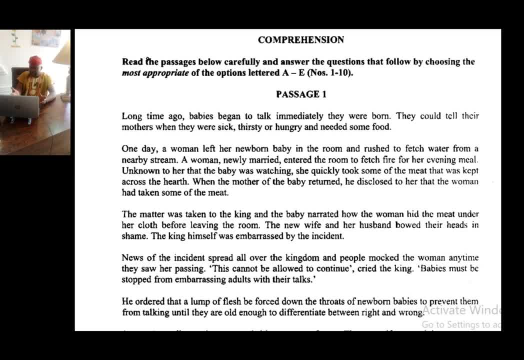 the foundation for success. Then it's also helpful, especially for comprehension passage, if you can read the question before you take or read the passage. It stimulates your mind And it makes it a lot easier for you to identify the answers in the passage. But for this, 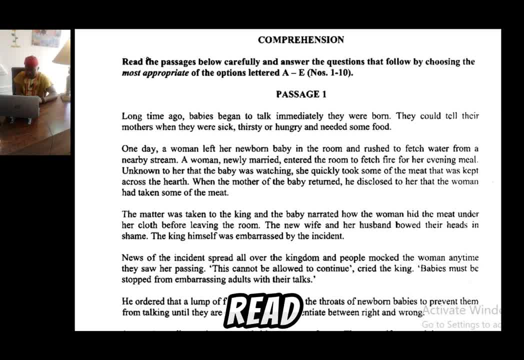 task. we're not going to read the question before we read the passage. Probably in the next class we'll do that. All right, so let's go on. Long time ago, babies began to talk immediately they were born. They could tell their mother when they were sick, thirsty. 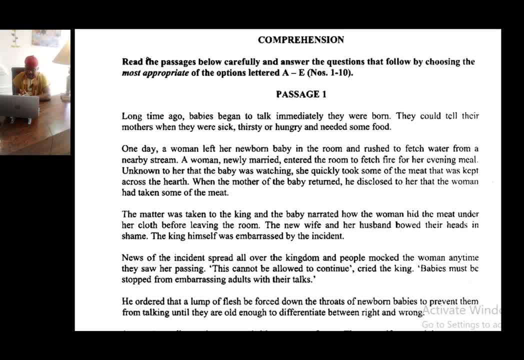 or hungry and needed some food. One day, a woman left her newborn baby in the room and rushed to fetch water from a nearby stream. A woman, nearly married, entered the room to fetch fire for her evening meal, Unknown to her that the baby was watching. she quickly 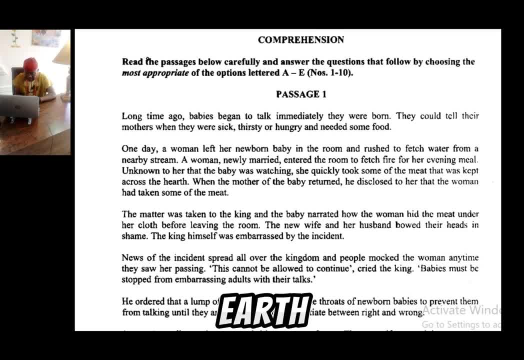 took some of the meat that was kept across the earth. When the mother of the baby returned, she heard a woman speaking. She disclosed to her that the woman had taken some of the meat. The mother was taken to the king and the baby narrated how the woman hid the meat. 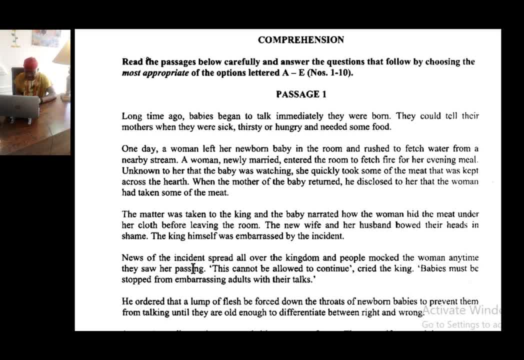 under a cloth before leaving the room. The new wife and her husband bowed their heads in shame. The king himself was embarrassed by the incident. News of the incident spread all over the kingdom and people mocked the woman any time she saw or they saw her passing. 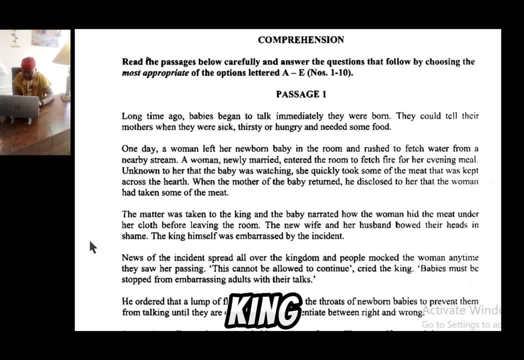 These cannot be allowed to continue. cried the king. Babies must be stopped from embarrassing adults with their talks. He ordered that a lump of flesh be forced down the throats of newborn babies to prevent them from talking until they are old enough to differentiate between right and wrong. 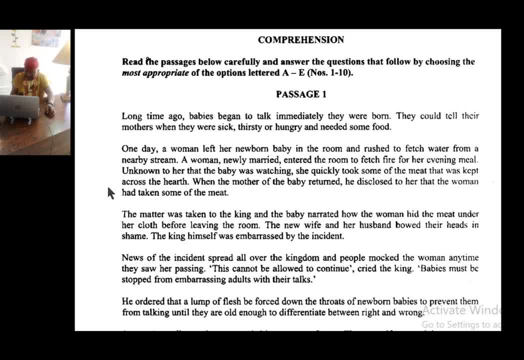 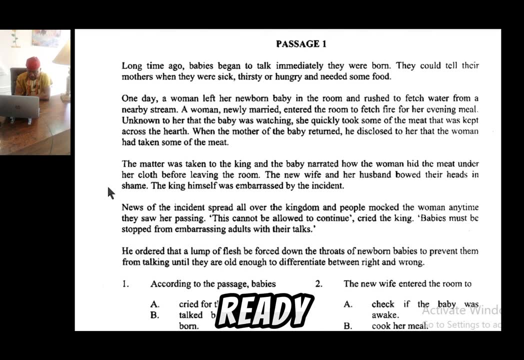 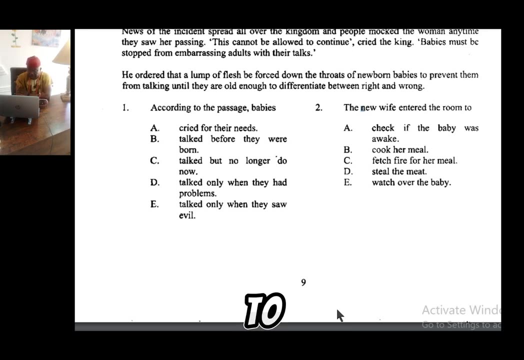 That's the passage. Hope you understood the reading. Now we are going to proceed to the question part. Really, To the questions now. Question 1 says: According to the passage, Babies. So we have to complete the sentence. Option A says: 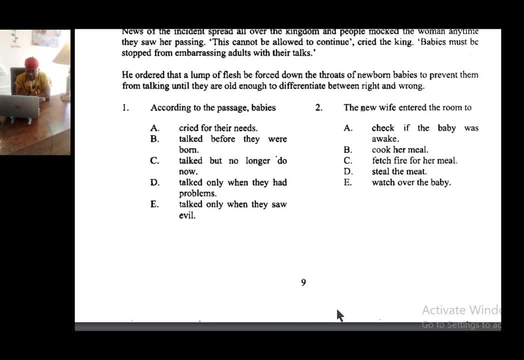 Cried for their needs. Talked before they were born. Talked, but no longer do now. Talked only when they had problems. Talked only when they saw evil. What do you think? the answer is: Of course we didn't hear about crying for their needs. 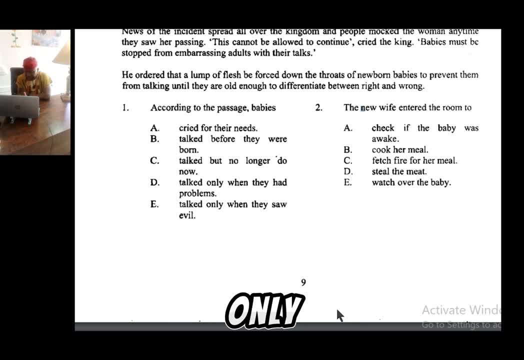 We didn't hear about talking only when they saw evil. That wasn't mentioned. So you can eliminate the wrong options. It makes it a lot easier for you to pick the right answer. So eliminate the wrong options first, Then you narrow it down. 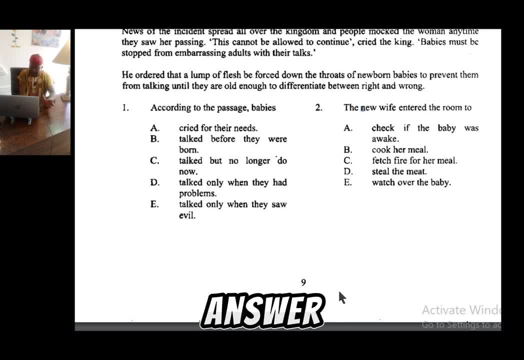 Then you narrow it down to probably the one correct answer and one wrong answer or wrong option. Of course it can be a wrong answer and wrong option. So talked only when they had problems Talked, but no longer do. now I think we can verify C because baby talked but after a while because of the incident. 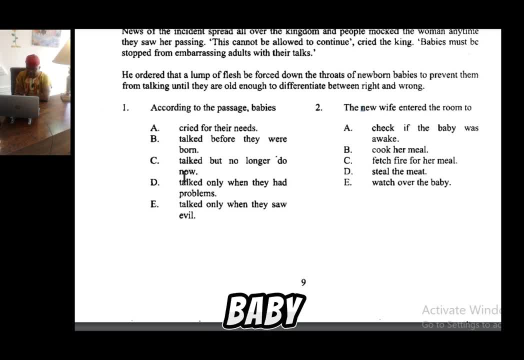 that happened. the king ordered that babies should not talk. Talk up again, as something was done about it. So that makes option C the right answer. Doalurgoq question to you, the new. I've entered the room to check if the babies were. the baby was. 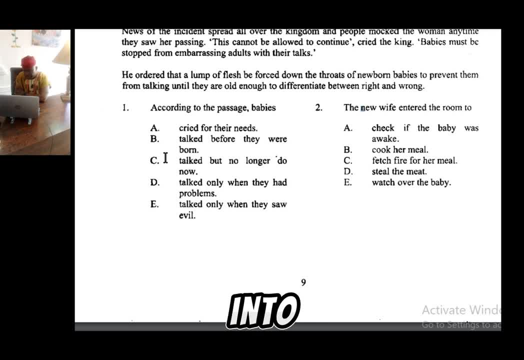 awake because I was not. why she went into the room. according to the passage B says cool a meal. That wasn't why she went to the Damn. it says cook a meal and the baby's not awake went to the into the room. option c says fetch fire, fire for a meal. 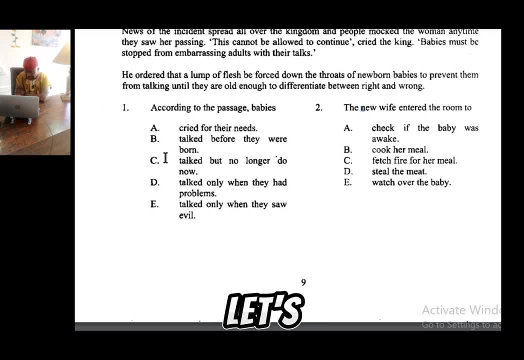 okay, that sounds like an option right, so let's leave it. steal the meat, otherwise she went into the room. okay, let's leave that too. watch over the baby. of course, that's completely wrong. so we have option c and d. it could be either of the two, so let's confirm from the passage: 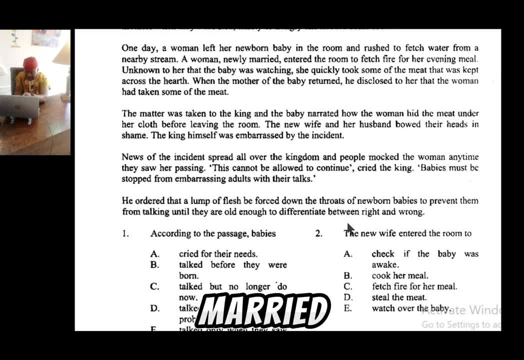 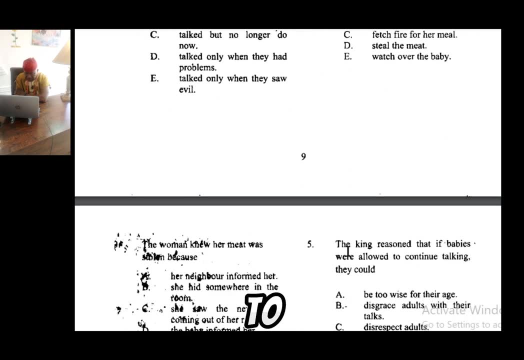 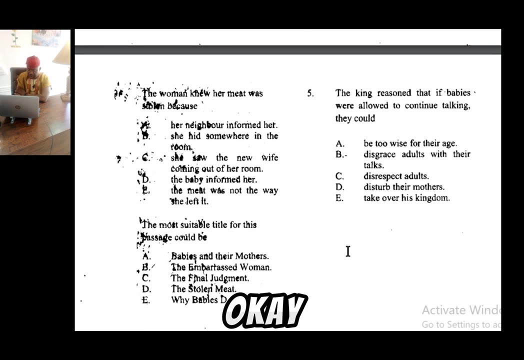 it says in a woman- nearly married- that's line two- enter the room to fetch fire for evening meal. so the clear answer is option what option c. so make progress to question three. okay, question three. pardon the blurriness in the typing, but i'll read it to make it a lot easier for. 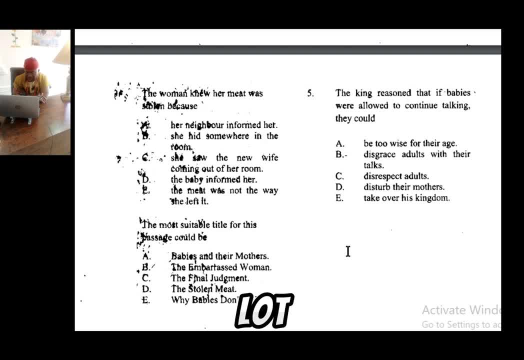 us to relate with. the woman knew her meat was stolen because her neighbor informed her that's not part of the passage she did. she hid somewhere and she was not able to find the meat in the room. that wasn't part of it, the information we got. she saw the new wife. 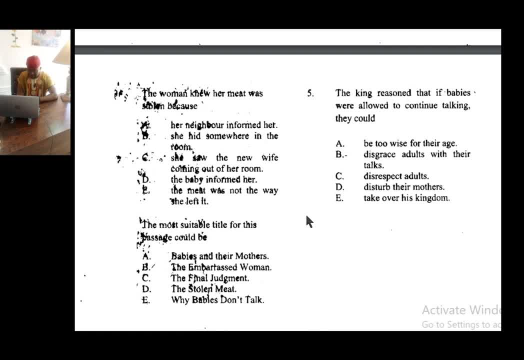 coming out of her room. that wasn't part of it too. the baby informed her. of course that is the answer, because we can prove that from the passage. so the answer is option d for number three. the most suitable title for these passage could be babies and their mothers. 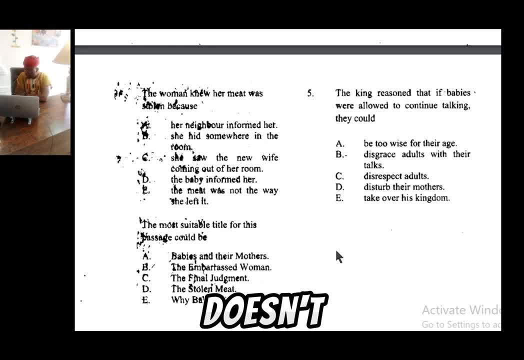 babies and their mothers. okay, it doesn't seem like an appropriate title for me. let's look at b, the embarrassed woman, the final judgment, that's option c. option d- the stolen meat, then option e: why babies don't talk? what do you think? your guess is as good as mine. 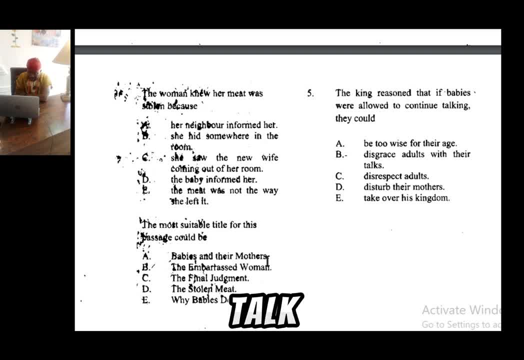 i think the answer should be e, because when you talk about title, it's encompasses the entire idea in the piece. so what is the essence of the whole story? from beginning to the end, it simply informs us why babies don't talk anymore, starting from what happened and the arrangement was chronological- how it happened and 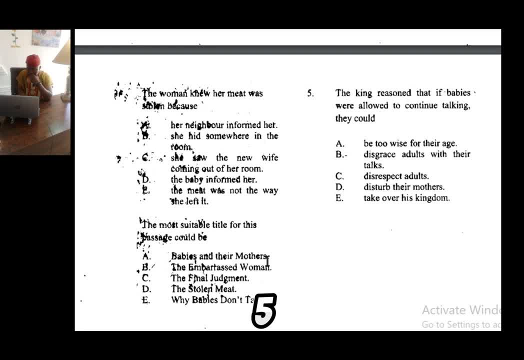 where we are right now, so go to question five. the question says the king reasoned that if babies were allowed to continue talking, they could a be too wise for their age. we can't prove that. disgrace adults with their talks. that sounds very much like the answer, option b, but let's look at. 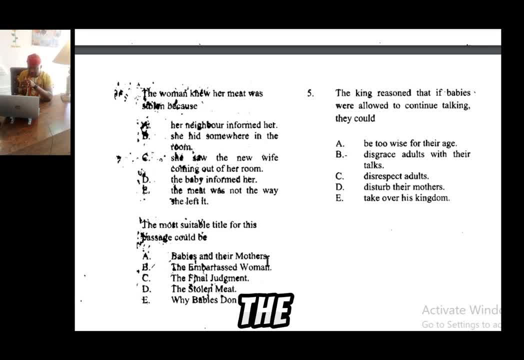 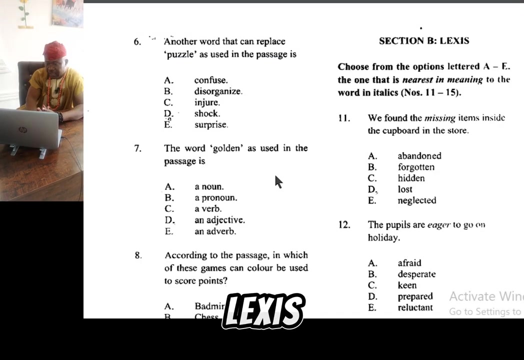 other options always good too. exhaust the options before you pick an answer. option c says disrespect adults. option d: disturb their mothers. option e: take over his kingdom. okay, having uh examine all the options, the most appropriate option seems to be option b: disgrace adults with their All right. so we go to Lexis section B, which is Lexis and Structure. 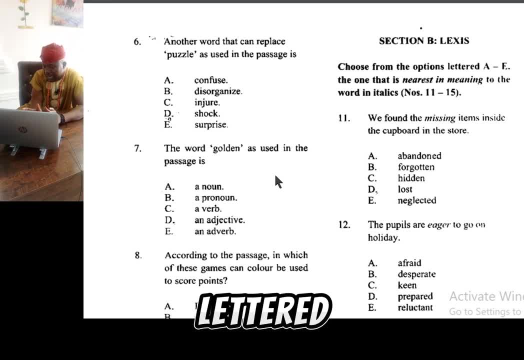 The instruction says: choose from the options letter A to E, the one that is nearest in meaning to the word in italics. So this is synonym. Now, one thing I've discovered is at times when you want to take this task, probably, 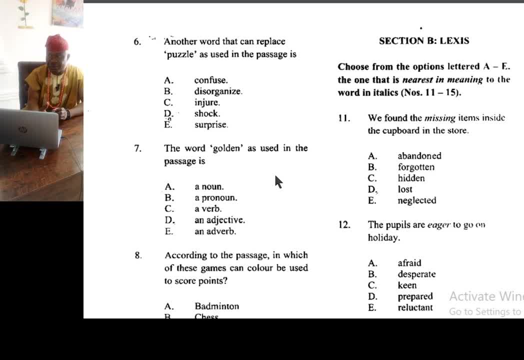 by default. it's human error. Most times, you just discover that, although we are supposed to pick synonyms, you're picking antonyms. It has happened to me several times Before I started doing something. what was it? as I read the instruction, I will mark. 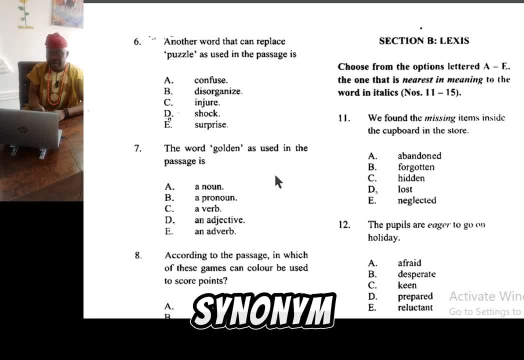 nearest in meaning or write synonyms. By that. it sticks in my mind that I'm working with synonyms, I'm picking synonyms So I don't go off plan. So question six says Another word. I can replace puzzle, as sorry Chris. question 11, that's where we're supposed. 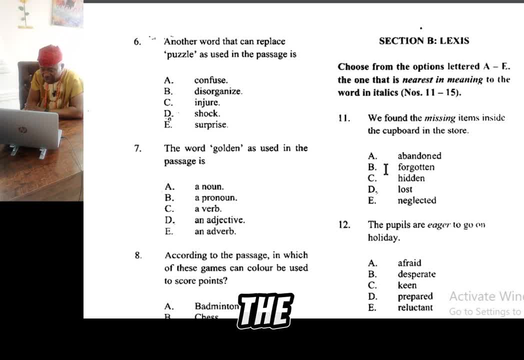 to start from. We found the missing items inside the cupboard in the store. Missing is it abandoned items? Is it forgotten item? Is it hidden items? Is it lost items? Is it neglected items? What do you think? I think the answer is lost. 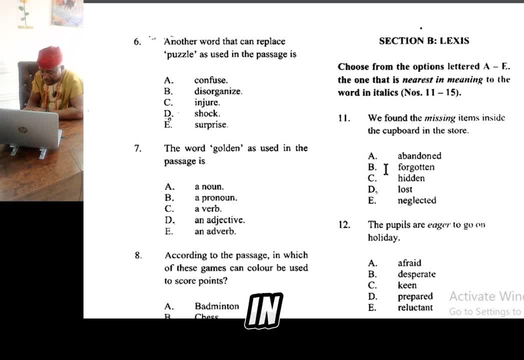 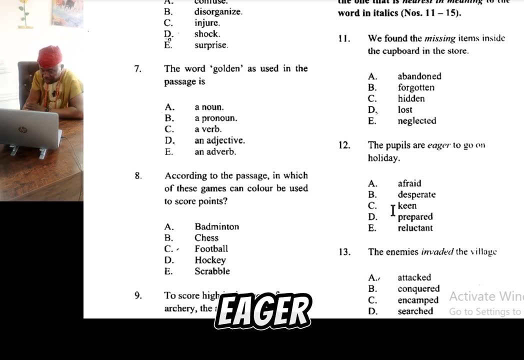 So we found the lost items inside the cupboard in the store. Question 12, The pupils are eager to go on holiday. The italicized word there is eager. Option A says afraid, B, desperate, C, scared, D, keen, D, prepared. 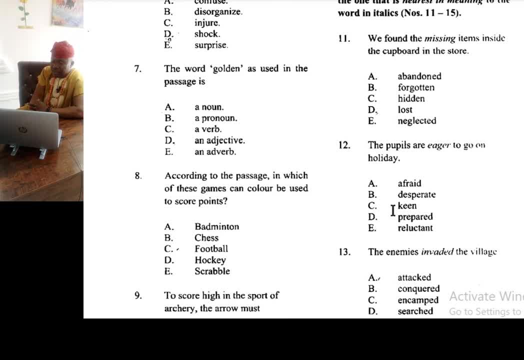 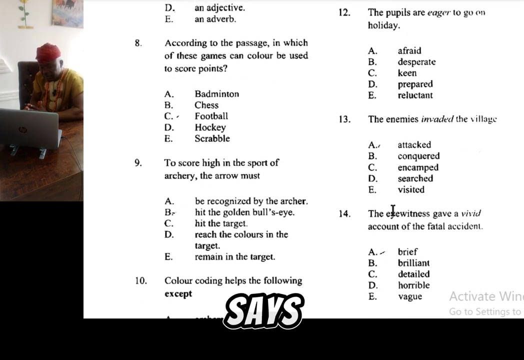 E reluctant, The answer should be keen. When you're keen on something, you want it so badly, So eager has the same meaning, especially in this context, And that authenticates C has correct answer. Question 13 says The enemies invaded the village. 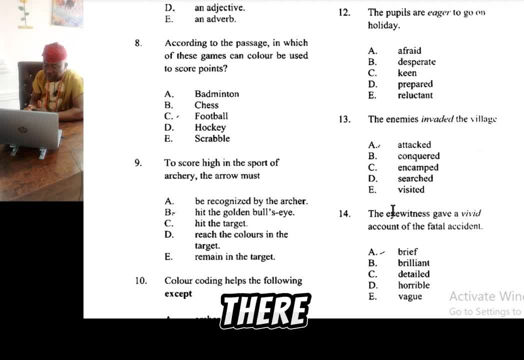 Question 13 says The enemies invaded the village. The italicized word there is invaded. Now let's go talk about using context clues here. There are times when, especially when it comes to vocabulary, synonyms and antonyms, you can't know all the vocabularies in an English language. that's just the truth about it. 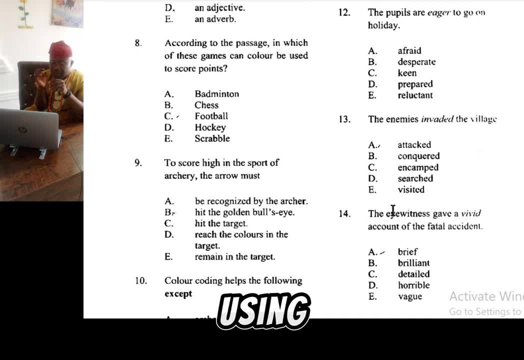 But when you're dealing with tasks like this, using context clues can help a lot. For example, in this question 13,, you have the enemies invaded the village. So even if you didn't know the meaning of invaded, but you have the enemies, then you have the village. 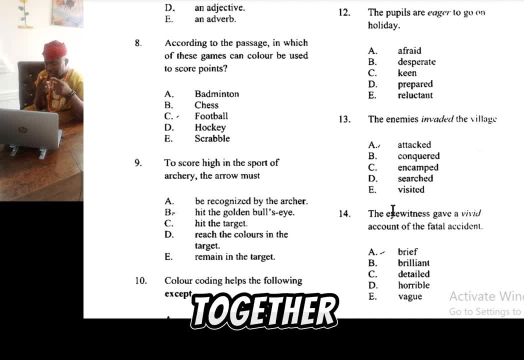 So you can put the dots together, you can connect the dots. What will an enemy go to the village to do So? invade or invaded will most likely mean what Attack. So using context clue, it can help a lot. So let's look at the options. 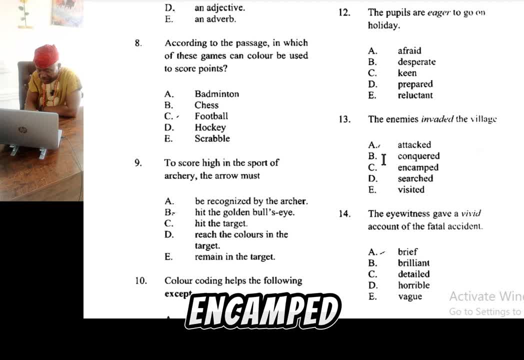 Attacked, conquered, encamped, searched, visited. The answer is attacked. The enemies attacked the village. Hope that helps. Question 14.. The eyewitness gave a vivid account of the fatal accident. Now eyewitness, like we discussed in question 13,. talking about context clues, 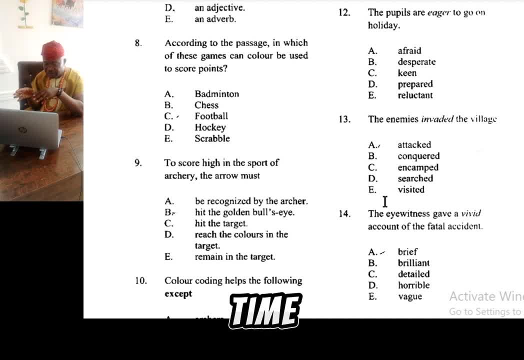 eyewitness is, someone who was there at the time of incident of the fatal accident gave a vivid account. So you can begin to put the dots together. What could vivid probably mean? Let's look at the options. A says brief, short. 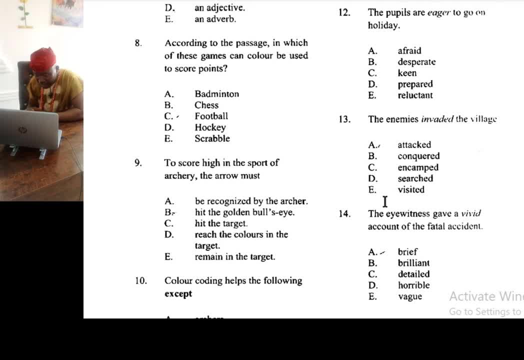 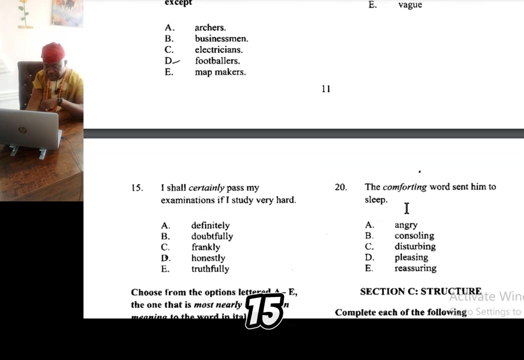 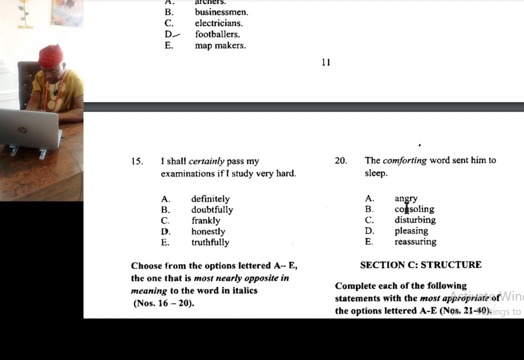 B says brilliant, D, C rather says detailed, D, horrible, E vague. The answer to this question is C, detailed. We go to question 15.. Question 15 says: I shall certainly pass my examinations if I study very hard. 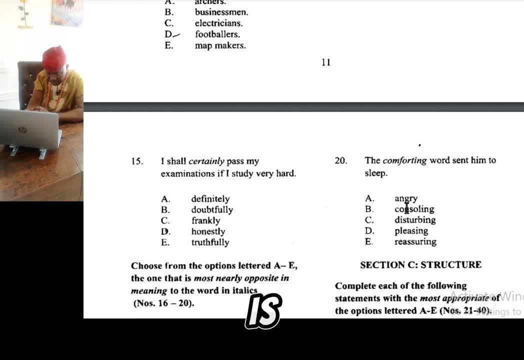 The italicized word is certainly. What about the options? Option A says definitely. I shall definitely pass my examinations if I study very hard. Option B says doubtfully. C says frankly, D honestly, E truthfully. What do you think? 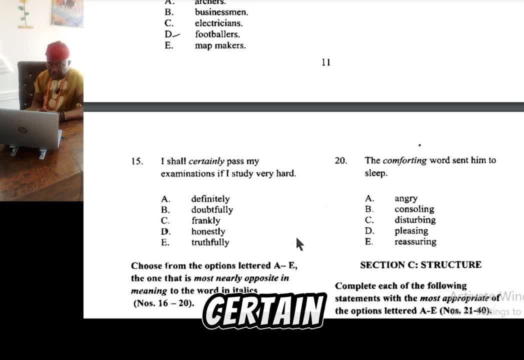 Certain, Are you sure? Are you certain, Are you definite? So the answer is definite A, I shall definitely pass my examinations if I study very hard. Okay, we're done with that. We'll make progress to questions 16 to 20.. 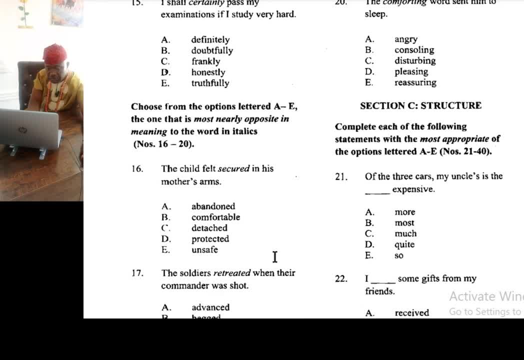 The instruction says: Choose from the options lettered A. Okay, so we'll go to the next questions, Questions 16 to 20.. The option says: Choose from the options lettered A to E, the one that is most nearly opposite. 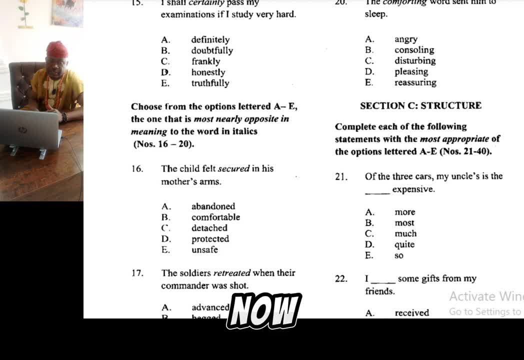 in meaning to the word in italics. Now, this is antonyms. All right, So let's get through it. Question 16 says The child felt secured in his mother's arms. The italicized word there is secured. Remember we are dealing with opposite. 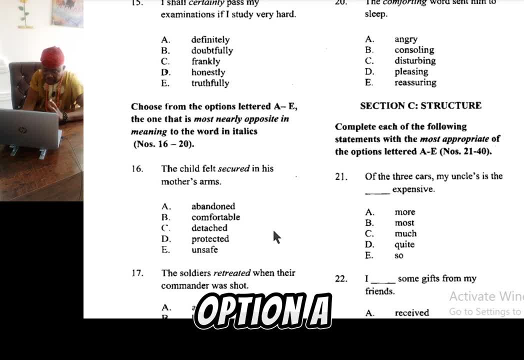 Abandoned. Option A. Option B: Uncomfortable. Go option C: Detached. Option D: Protected. Option E: Unsafe. What do you think is the opposite of secured Is unsafe. So the answer is option E. We go to question 17.. 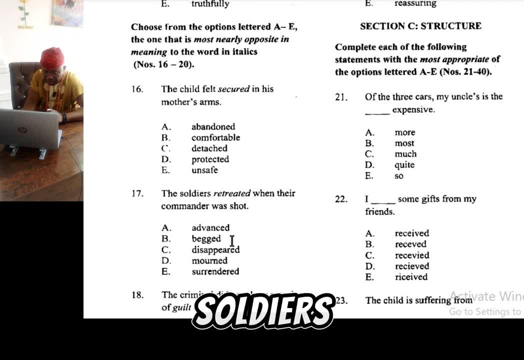 The soldiers retreated when their commander was shot. The soldiers retreated when their commander was shot. What is the opposite of that Option? A, Advanced, B, Begged, C Disappeared, D Mourned, E, Surrendered. 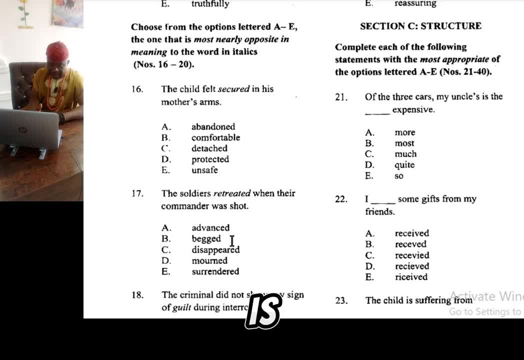 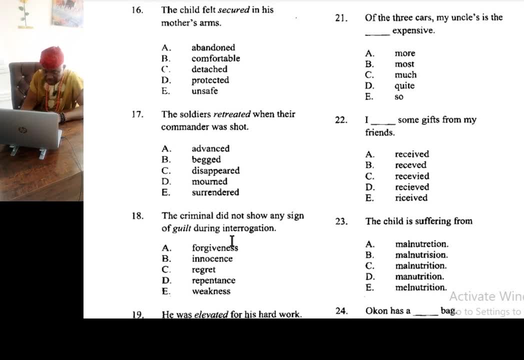 What do you think? The answer is A Advanced Question 18.. The criminal did not show any sign of guilt during interrogation. The italicized word is guilt. So what is the antonym? Forgiveness, Omniscience, Innocence. 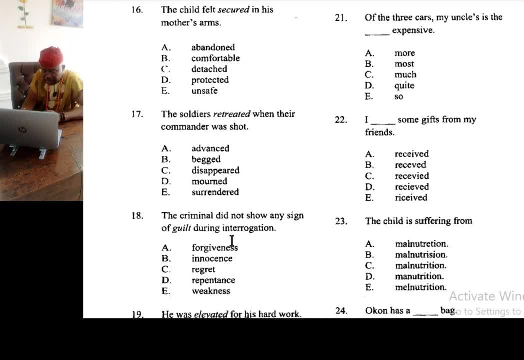 Regret, Repentance, Weakness- What do you think the answer should be? The answer is repentance. That's the opposite of guilt, Repentance, And that is option D. The criminal did not show any sign of guilt during interrogation. 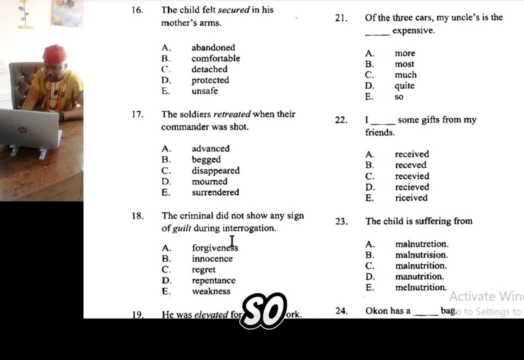 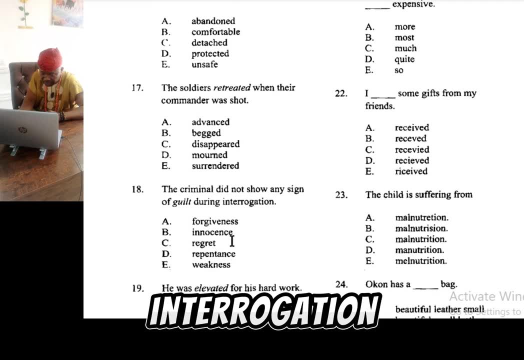 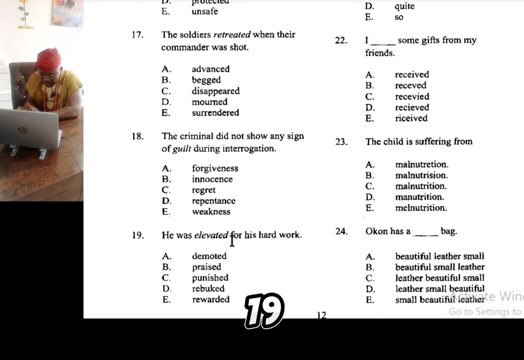 The italicized word is guilt Persecution. so the criminal did not show any sign of repentance during interrogation. all right. question 19: the question says he was elevated from his hard work. option a, first of all. the italicized word is elevated. now option a says demoted, b pressed, c punished, d rebuked, e rewarded. 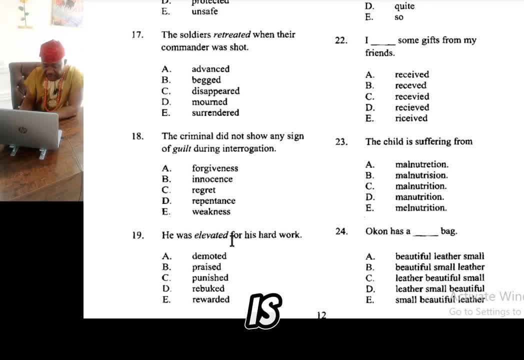 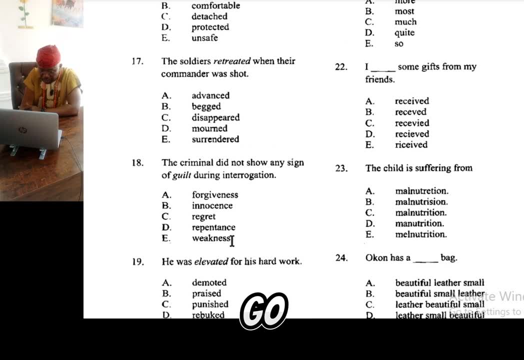 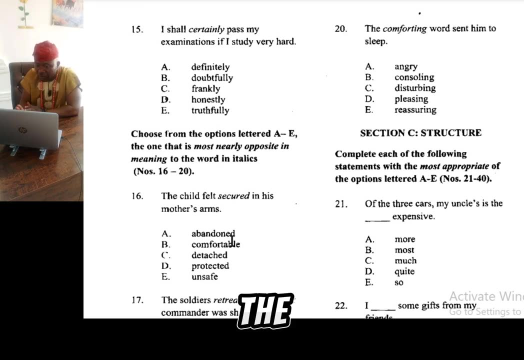 what do you think the answer is? the answer is demoted, elevate, demote. we go to question 20.. question 20 says the comforting word sends him to sleep. the italicized word is comforting. what is the opposite of comforting? option a: angry, b, consoling, c, disturbing, d, pleasing, e, reassuring. 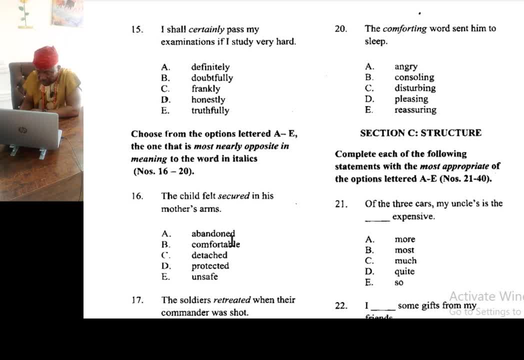 what is the opposite of comforting. it should be option c, which is disturbing. all right, so we're done with that section. we're going to section c, which is structure. the instruction for section c says: complete each of the following statements with the most appropriate of the options lettered a: 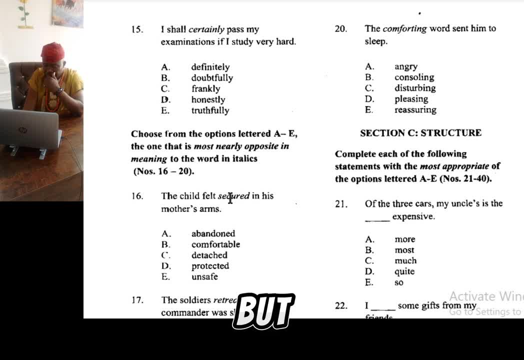 to e, but then with numbers 21 to 40.. question 21: one of the three cars- sorry, of the three cars, my uncle's- is the dash expensive. now, what's the answer here? the right answer is b, which is most. what is the reason? you're comparing three and that takes you to the superlative. 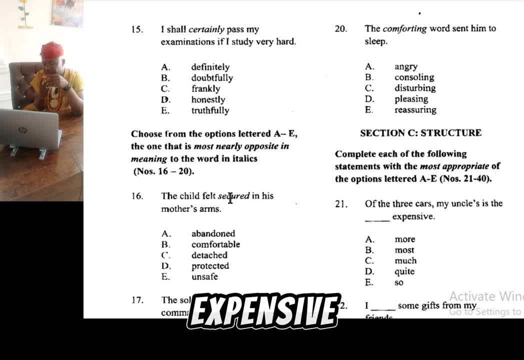 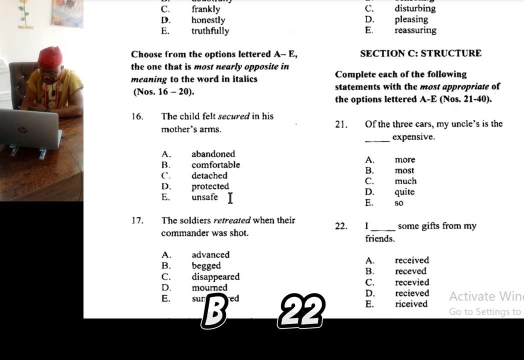 comparison and the superlative comparison of expensive, because expensive is more than one or two syllables and once you have more than two syllable words or adjectives, it takes more for comparative and take most for superlative. so the answer is b 22. i dodge some. 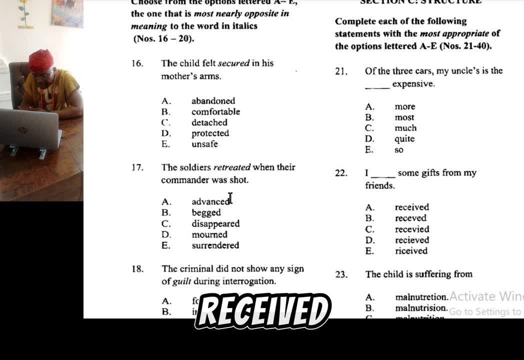 gifts from my friends. i don't have any gifts from my friends. i don't have any gifts from my friends. that is a bot, Bronx Europe, which gives us b 12 and seven. right, we have been given b eight. so i don't have much income, but i i'm NOT going to choose be. 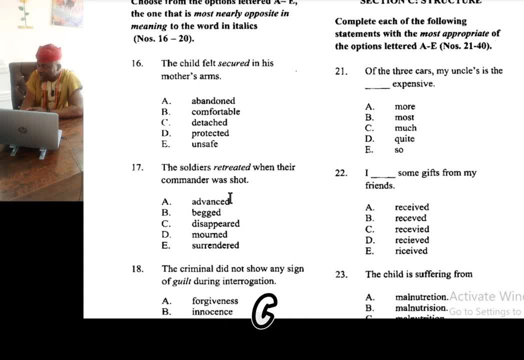 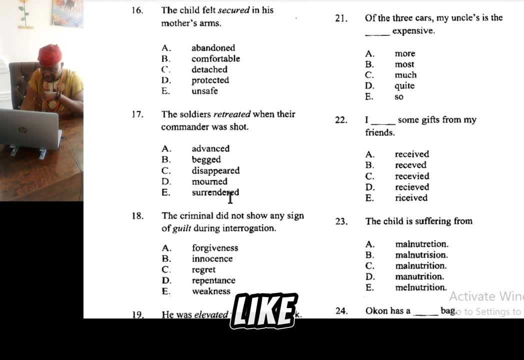 returns either in the navy or inappropriately, or in d jeffries which is is going to give us with EXuteness so we can enter in that description. the answer is a, but the answer is: let me see what's Freeze let'sосьue. 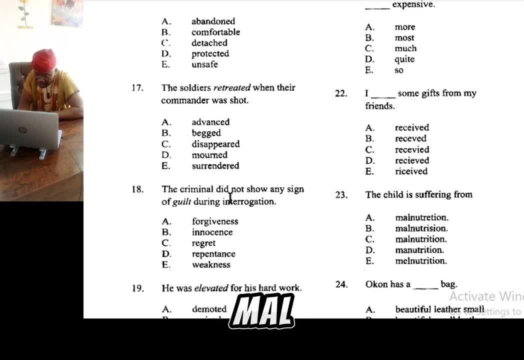 retrieve received. ask Mal M-A-L. Then you have okay. look at option C: M-A-L- malnutrition. Although you have the confusing part, here is the shown part. There are some words that end with S-I-O-N. 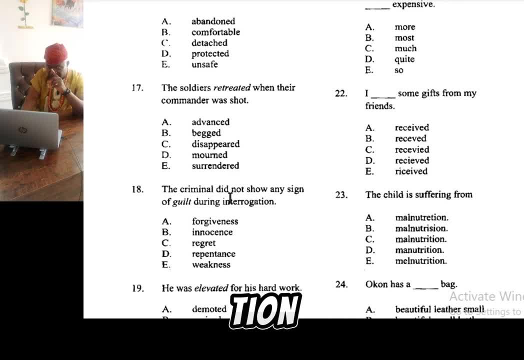 and they sound shown. and some still end with T-I-O-N and still sound shown. So you need to familiarize yourself with these word endings to scale questions like this. But for this particular question the answer is option C. Malnutrition is spelled M-A-L-N-U-T-R-I-T-I-O-N. Thank you. 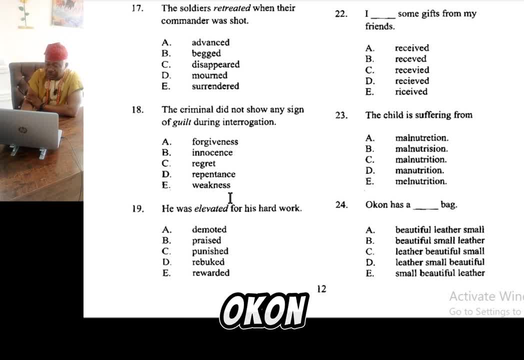 We go to question 24.. Question 24 says Ocon has a dash bag. Now, if you notice, we have three adjectives after one another. Now what this is testing is what is called order of adjectives. Order of adjectives. So what does that mean? It? 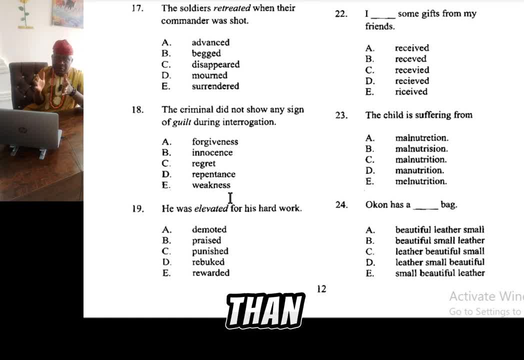 means that you want to describe something and you have more than one adjective to describe. So, like we were saying, order of adjectives is when you have something you want to describe and you have more than one adjective to describe that particular thing, probably because of 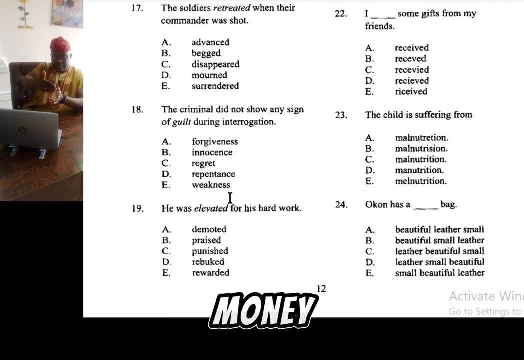 how fantastic it is. There is a mnemonic that helps you order or arrange the adjectives, because you don't just, you know, dump the adjectives. there It's called: you know, sascomp, You know sascomp. Okay, probably one of our classes will treat that separately, so that 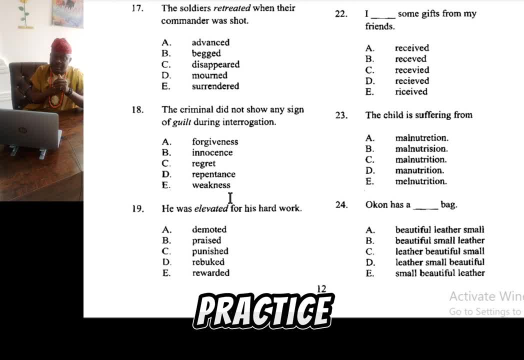 you can, then you know, give you practice. You know practice, practice, practice, practice, practice practice, And then you can ask questions on it so that you can become quite familiar with it, Now that nosascomp is a mnemonic that helps you understand how to. 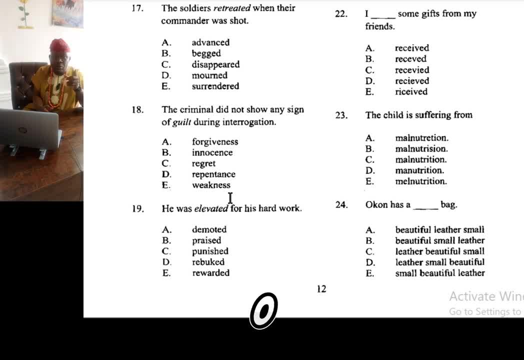 arrange the adjectives: N stands for number, O stands for opinion, S stands for uh size, A stands for age S. the second S stands for shape, C stands for color, O stands for origin, stands for material, then p for purpose. so that's no sascom. so if you look at that, 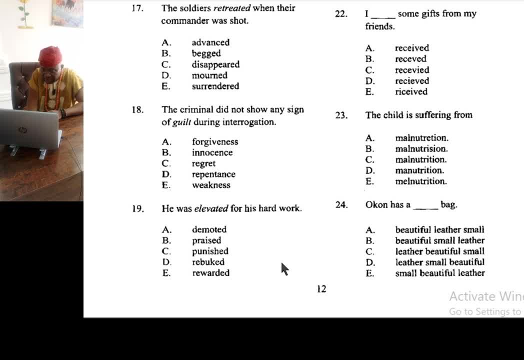 there are three adjectives here. beautiful, first, the first: uh, our order is number, so we don't have number here. but the second one is opinion. remember, it's no. so the second is opinion. do we have opinion here? what's your opinion of this bag? the opinion is that it is beautiful. so that automatically eliminates option c, d and e. 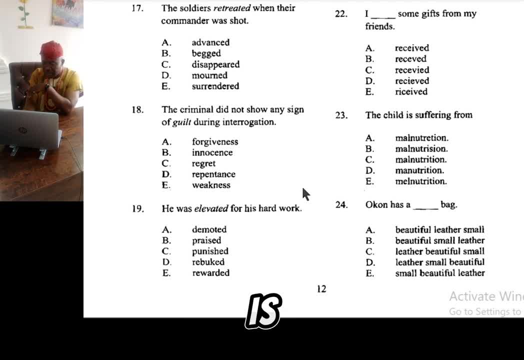 so we're between a and b. beautiful is our opinion of the bag. okay, what's next? no, that's opinion s shape. do you have shape? no, do we have, no, sorry. the next one is size. do we have size? after beautiful in a and b? for a, we have leather, which is material. 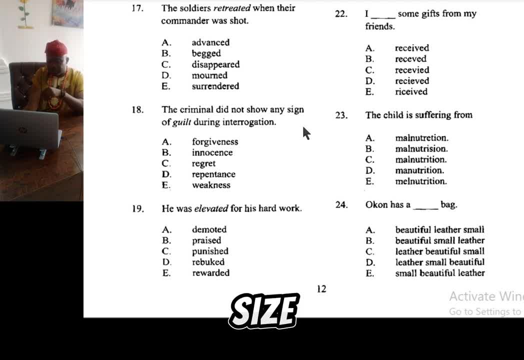 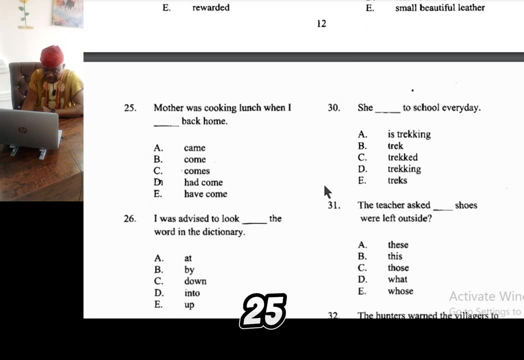 but for b we have small, which is the size, so that automatically makes option b the right answer. so, like i said, watch out for a class on other objectives. so that you can familiarize yourself with that concept, we go to question 25. question 25 says mother was cooking lunch when i dash back home. 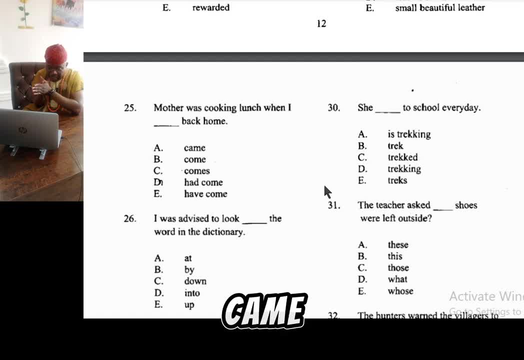 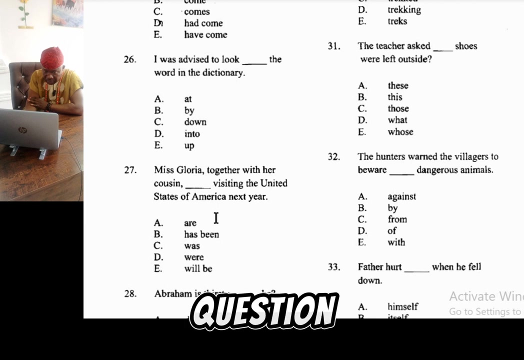 mother was cooking lunch when i came back home. that is option a. this is testing verb tense. go to the next question, which is question 26. question 26 says: i was advised to look dash the word in the dictionary a. i was advised to look dash the word in the dictionary. i was advised to look dash the word in the dictionary a. 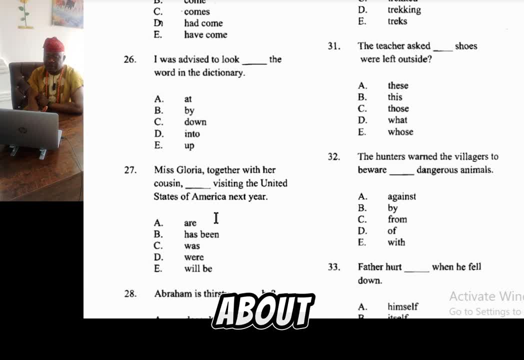 this is an example of colloquials. now, when you talk about colloquials, what does it mean? it means there are some words in english that you use together. they're used together, they're like, they're like a team, what people generally call five and six. so if you use this, you must use this. 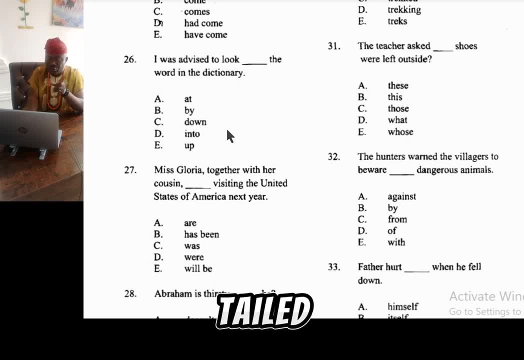 some of the colloquials in english are too tired: two, two and two, that's t-o-o and two, so you can say i'm too tired to sing, then so, and that i'm so tired that i can't. so in this case, what do you do? 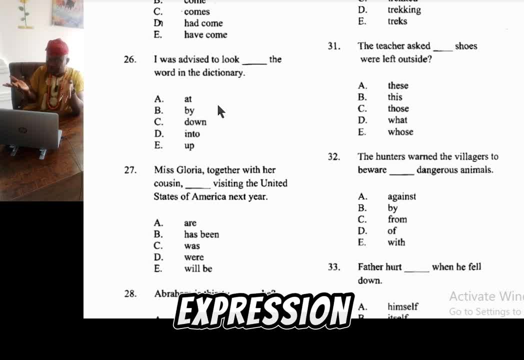 you look up a word in a dictionary. that's, that's the expression, that's how you use it. you say: you look at a word in a dictionary, okay, that sounds, you know, very acceptable. most people will probably jump at: uh, option a, but it's the wrong one. i guess that's how they kept it. 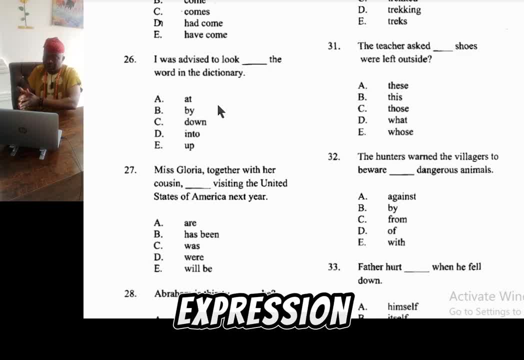 in the first option to mislead the out. but you look up an expression in a dictionary if you're not familiar with that, the meaning of the expression. so the answer is e question 27: miss gloria, together with her cousin dash, visiting the united states of america next year. now, together with her cousin, is a prepositional phrase. 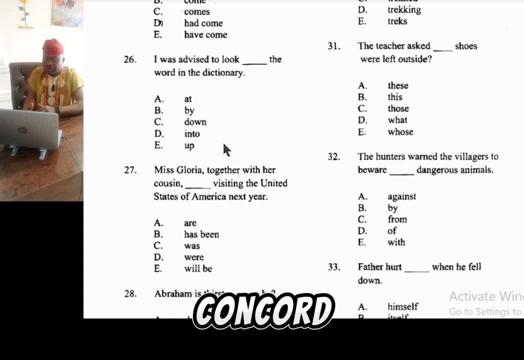 and this is testing concord, which is subject and verb agreement. in this sentence, the extra information, which is together with her cousin, does not change the number of the subject. the number of the subject remains singular because you're talking about one person, gloria. so the verb that you're going to choose must also be a singular verb. and if you look at the 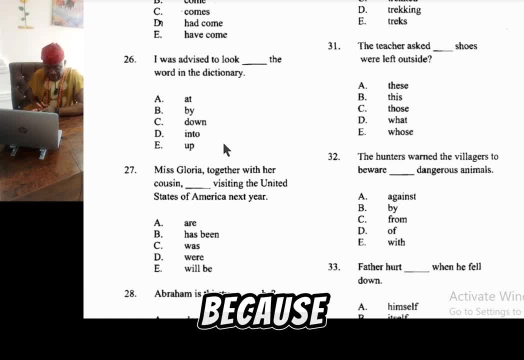 letter e and the sentence mbc. yours are the one that are liked. one, yes, ok. and e. the one that we need to consider is what is, or from which electrician could be speaking next year. so you see, that's the answer, um gloria. first one is: why didn't they? dough was fine, which was. 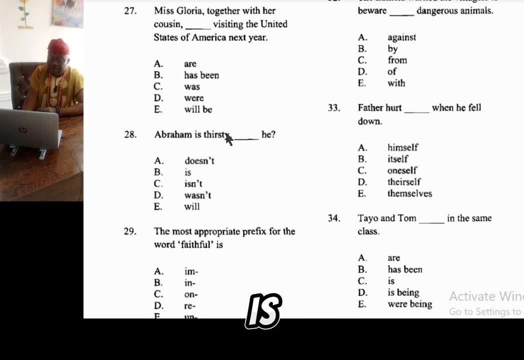 that they actually give them water in Да. of course she spent that money, but now she already want to to drink water again. now she only want water to get by. who else should she talk to exactly? because that's too errors, as she just talked about adonis. additional year and that is disease. when she is in the UK next year, which makes option e makes option e takes note of because r has been will not fit because we were talking about next year and that makes the plan futuristic, which makes option e the most appropriate. so the answer would be e and the sentence is: miss gloria will be visiting the united states of america next year, 28.. 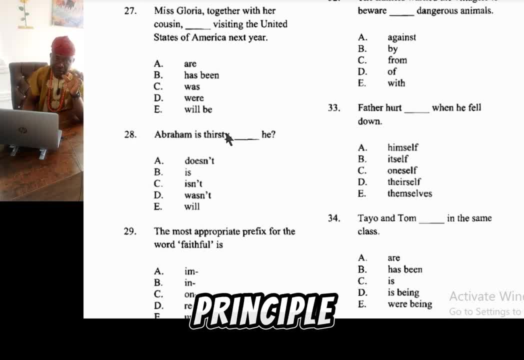 now this is question tag. question tag has a very simple principle: if the statement is positive, the question tag will be negative. if the statement is negative, the question tag will be positive. that's the simple rule that governs question tag. so if you look at this statement, abraham is thirsty is a. 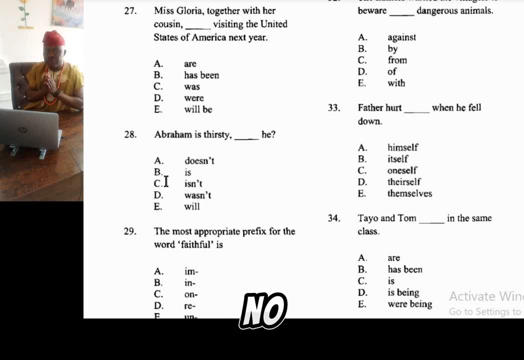 positive statement because there is no, not there and we don't have another negative word. we only have the subject, the linking verb and the predicate adjective, which is describing the state of being of abraham. so what is the question tag, since the statement is positive? abraham is thirsty. 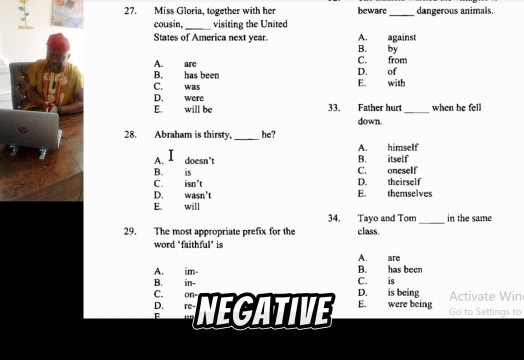 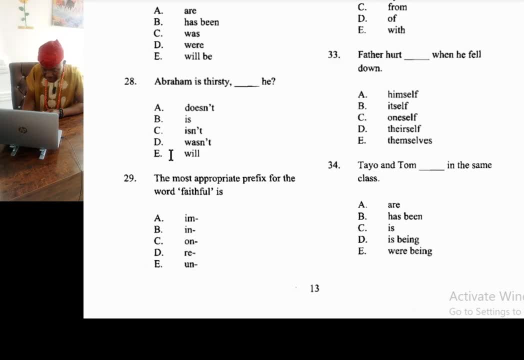 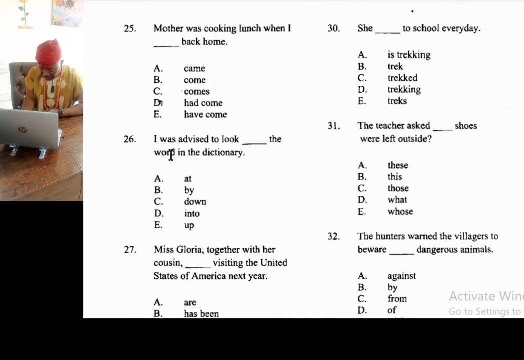 isn't he, the isn't there is a negative word, the not is a negative word. so the answer to that question is c. question 29. question 29: the most appropriate prefix for the word faithful is, of course, e. is the answer unfaithful? we go to question 30.. question 30 says she dashed to school. 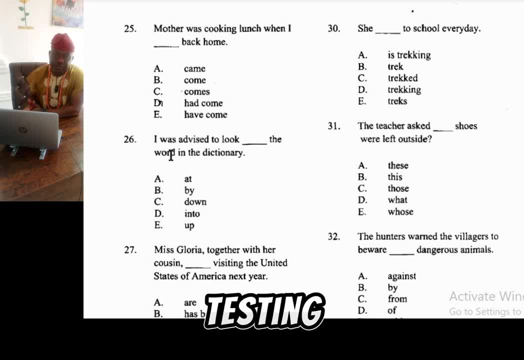 every day. now, this is testing verb tense. the simple present is used for continuous action. when i say continuous action, continuous action, i do not mean ongoing action. it means action that happened on a continuous basis. that's what is a simple present for. like i track to school every day. i eat because i do it. 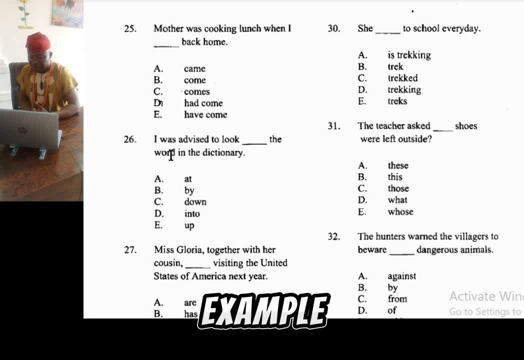 every time. so this is an example of that, and the option that fits the sentence perfectly is option e. she treks to school every day. it's a regular thing for her. Question 31,. the teacher asked whose shoes were left outside. Now you need a possessive here and the answer is E. the teacher asked whose shoes were left. 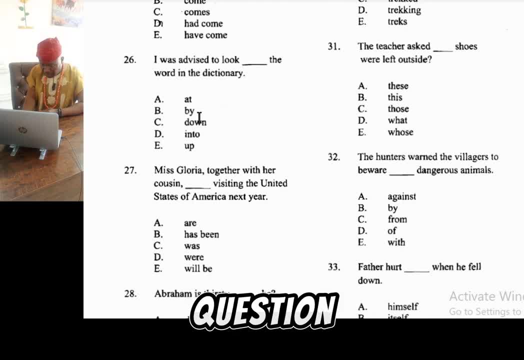 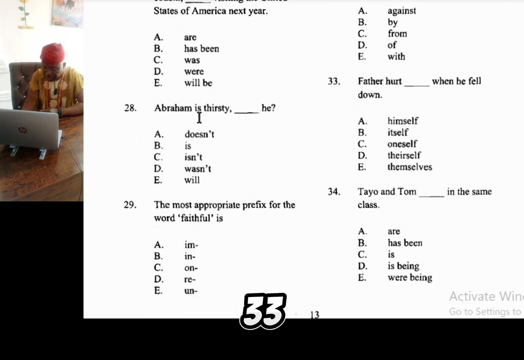 outside. Question 32, the hunters warned the villagers to beware those dangerous animals. You have to beware of dangerous animals. So the answer is D, to beware of dangerous animals. Question 33, father hurt Dash when he fell down. This is reflexive pronouns. 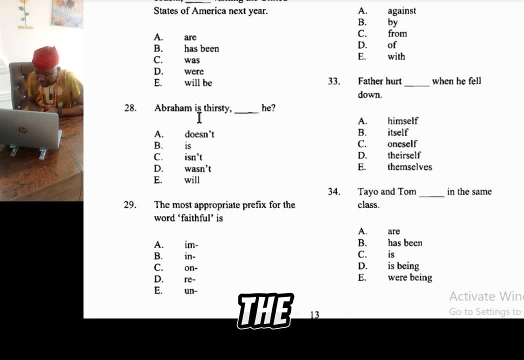 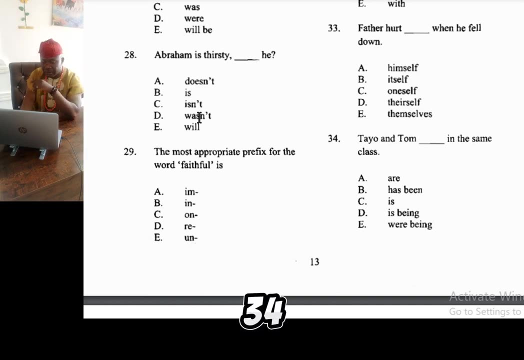 So, father, what should be the most fitting reflexive pronoun for father? there It should be himself. So father hurt himself when he fell down. The answer is option A. Question 34, Tayo and Tom dash in the same class. 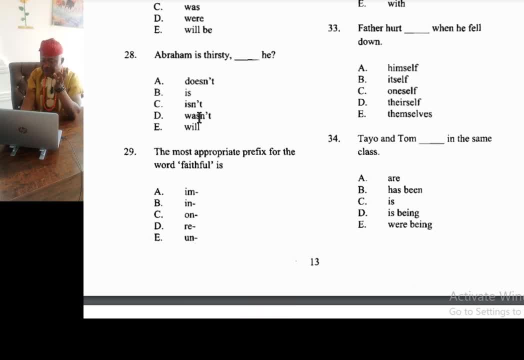 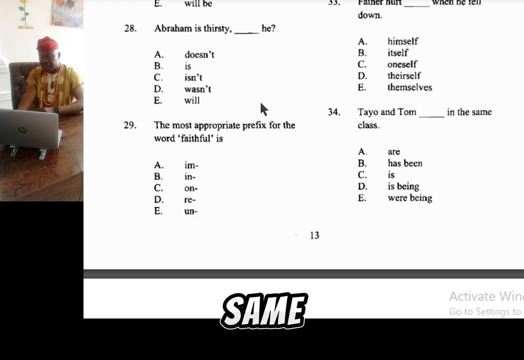 This is, to an extent, subject and verb agreement. Tayo and Tom. the subject is Tayo and Tom and it's plural subject, so you are required to use a plural verb in this class. Tayo and Tom are in the same class, So that makes option A the correct option. 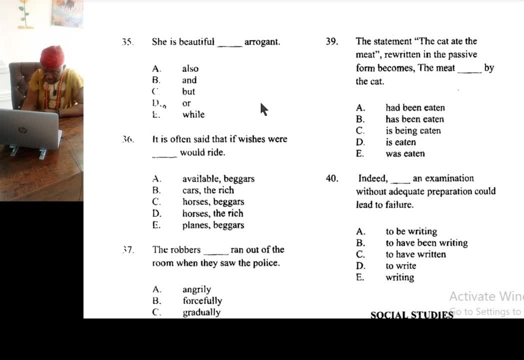 We go to question 35.. Question 35 says: she's beautiful, dash arrogant. Okay, now, this is the use of conjunction. she's beautiful, That's it. That's a good thing, that's a sweet thing. Arrogance is not a sweet thing. 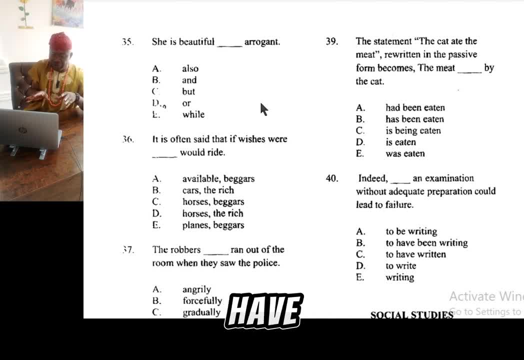 Arrogance is a negative trait. So we have two contrasting ideas here. and what conjunction do you use to show contrast? You use, but to show contrast. So you say she's beautiful but arrogant, because the arrogance will not complement a beauty. So the answer is C. 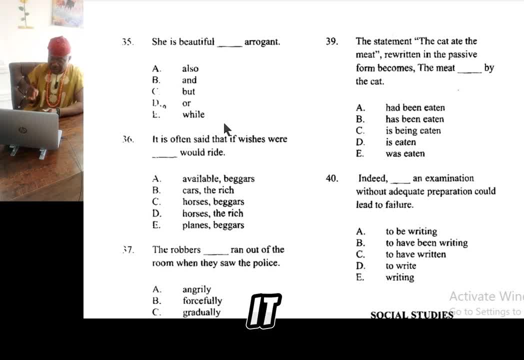 Question 35.. It is often said that if she wishes- sorry, if wishes were, were what- This is a. this is like an idiom: If wishes were horses, beggars would ride. So it's it's a long standing saying in English language. it simply helps us understand how. 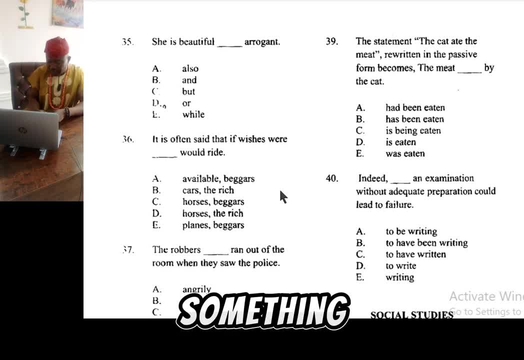 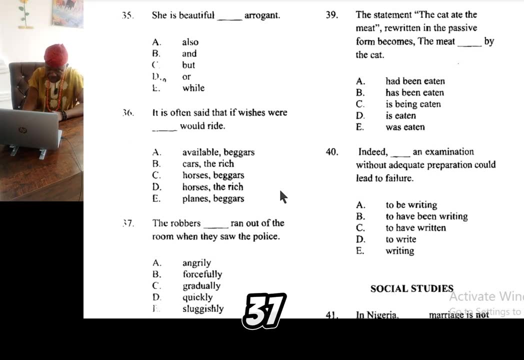 easy it is to make a wish for something. So don't just wish. go beyond wishing, Put actions behind your wish, and that's when your wish will come true. So that's what it's simply saying. Question 37. The robbers ran dash. okay, sorry, the robbers dash ran out of the room when they saw the. 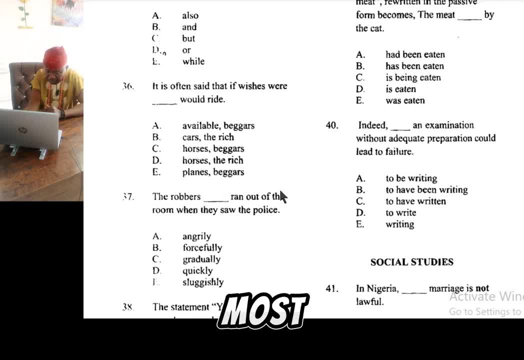 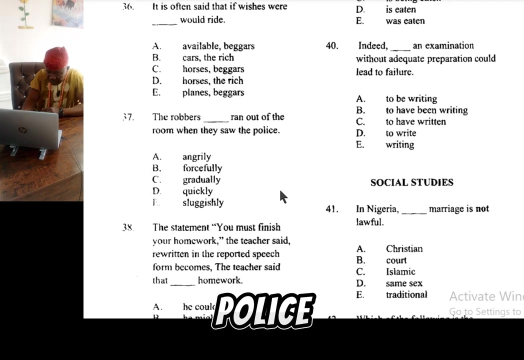 police. Okay, well, as you pick the most appropriate adverb, of course it can be angrily, it can be forcefully, gradually, because police is coming. So they can be sluggish about it. So they must have quickly run out of the room when they saw the police. 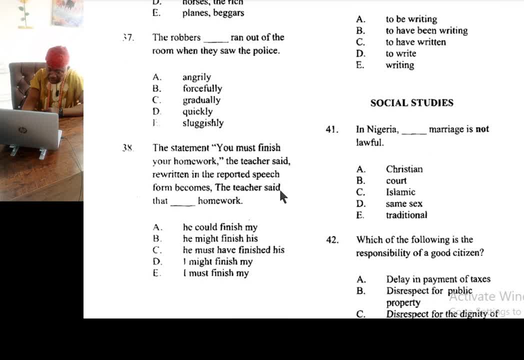 So the answer is D, Question 38.. Excuse me Question 38.. What is the statement? You must finish your own work. The teacher said we've written in the reported speech form becomes. the teacher said that he could finish my no. he might finish his no, he must have finished. 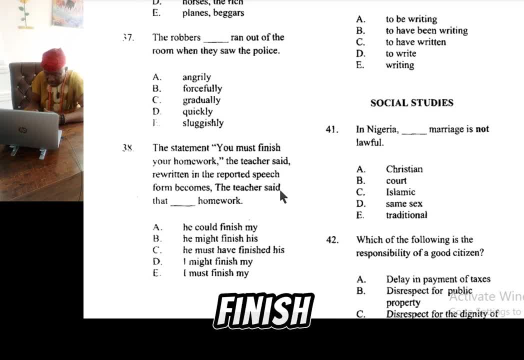 Question 39.. I might finish my. I must finish my okay homework. So the teacher said that I must finish my homework. The teach the statement you must finish your own work. the teacher said in reported speech would be. teacher said that I must finish my homework. 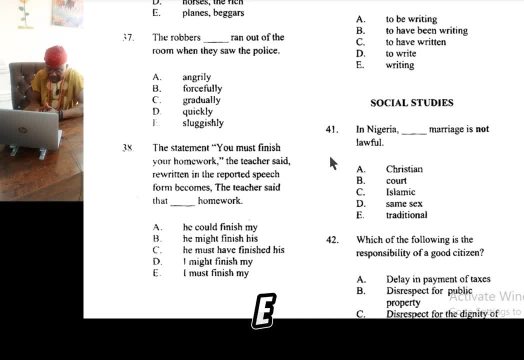 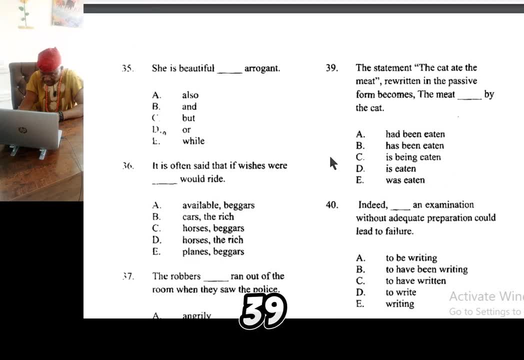 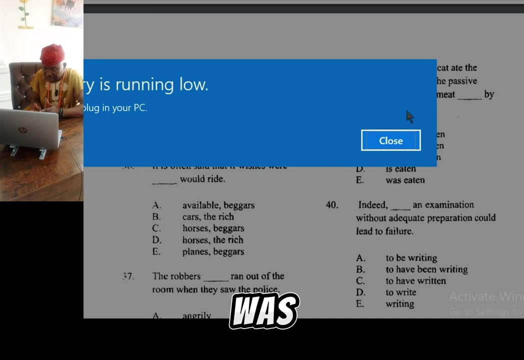 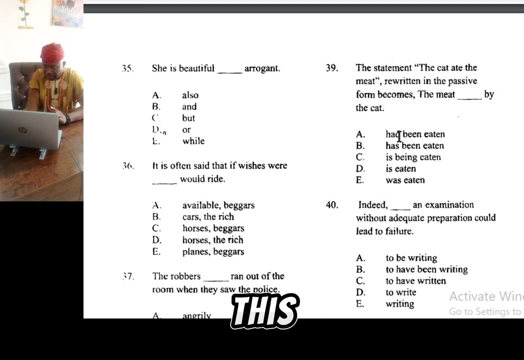 So that makes option E, Question 40.. Question 41.. The cat ate the meat, question 31.. He agreed The right answer. Question 39.. heart now talking about subject and verb. uh, this is a passive and active voice. we will have a video. 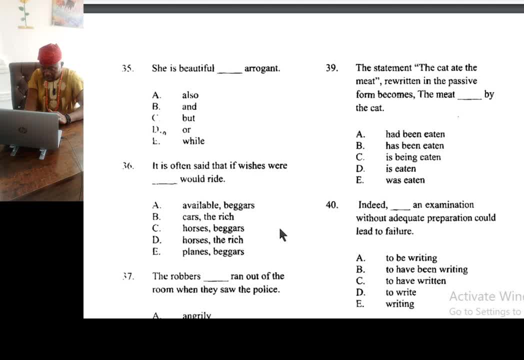 that will treat the rule comprehensively so that we become, you know, familiar with these grammar topics. question 40, which is the last question you've done. well, same thing till this time, okay. question 40 says, indeed, dash, an examination without adequate preparation could lead to failure. indeed, write an examination without adequate preparation.